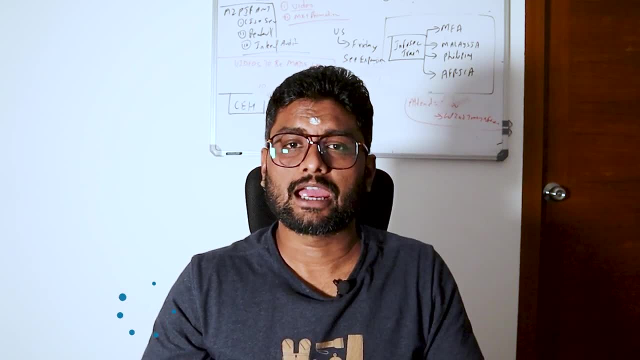 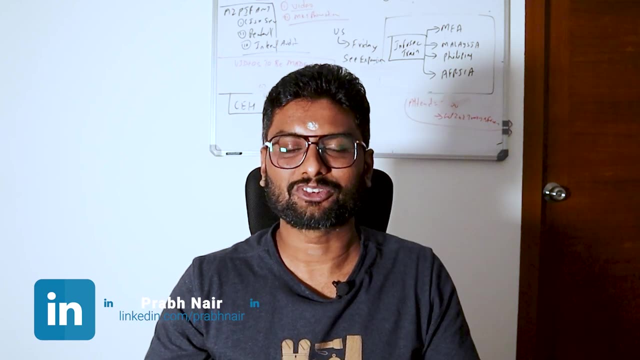 to make sure you should not miss my similar kind of videos in the future. And my name is Prabh Nair. for more information, you can refer my LinkedIn profile. So, without wasting a time, let's start with the first part. Hello everyone, my name is Prabh Nair and I'm working as a Chief Instructor. 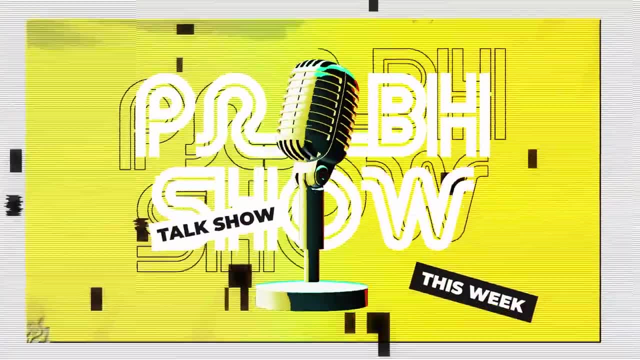 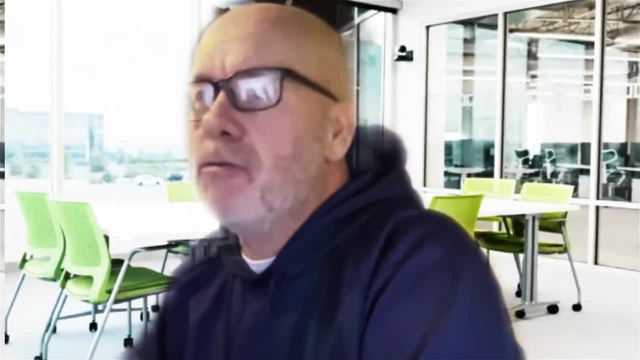 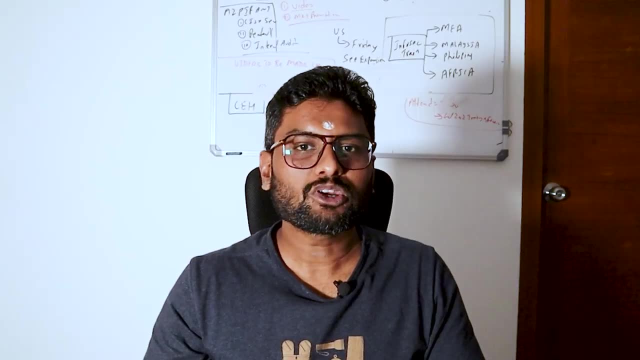 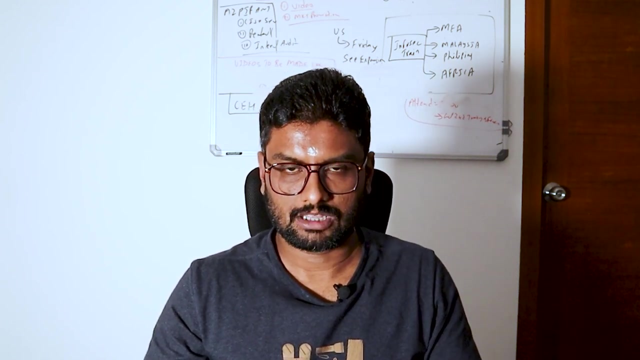 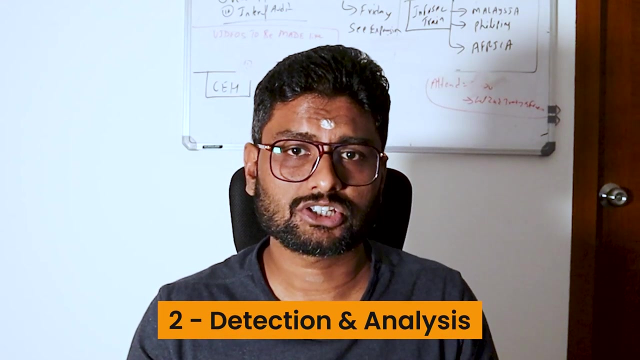 at Infosec, So when we're talking about incident management process. so incident management process is basically divided into the four stages. They have four stages. The first part, or first stage, is called as a preparation. The second part called as a detection and analysis. The third 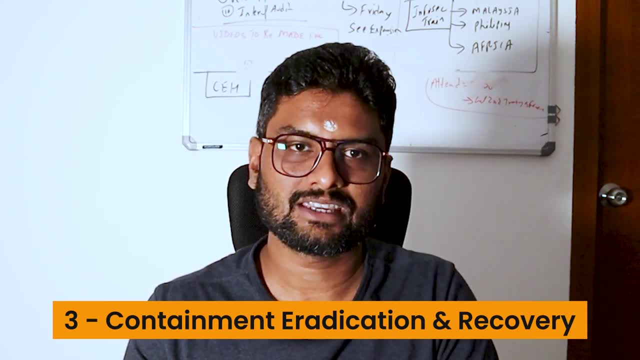 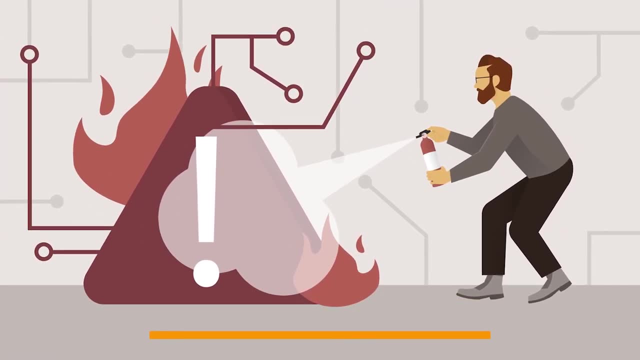 step, or third stage, is called as a containment, eradication and recovery. The fourth stage, or fourth step, is called as a post incident activity. So these are the four steps we have, or four stages we have, So when we're talking about incident management, 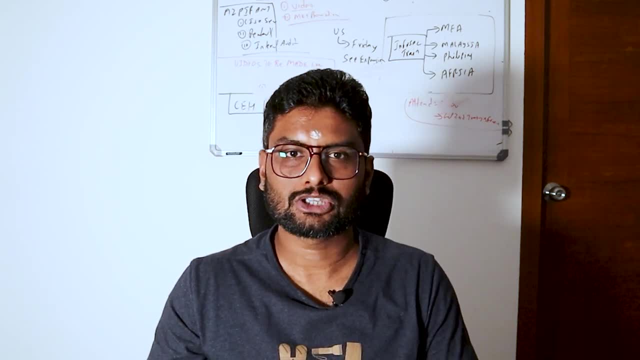 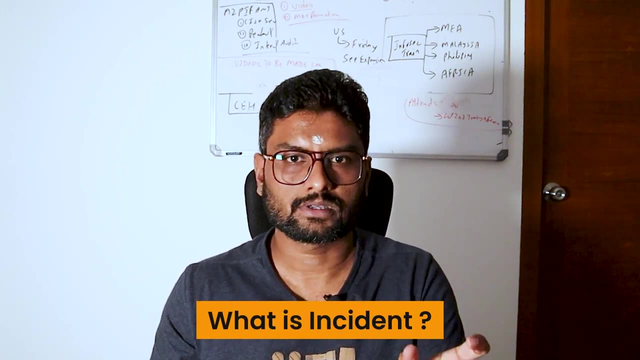 process. the ultimate goal of the incident management process is to reduce the impact. always remember. But before going to understand the stages in detail, let's understand what is incident. So, if you go by the definition, incident is any series of activity which impact. 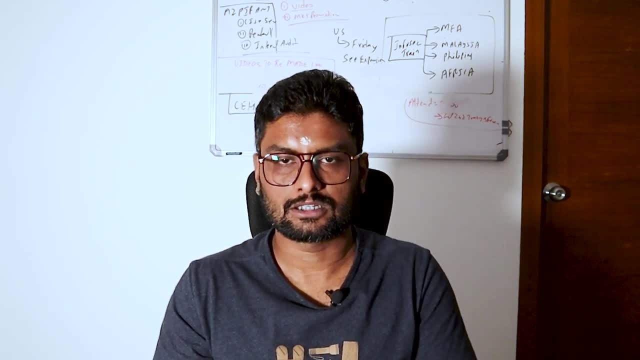 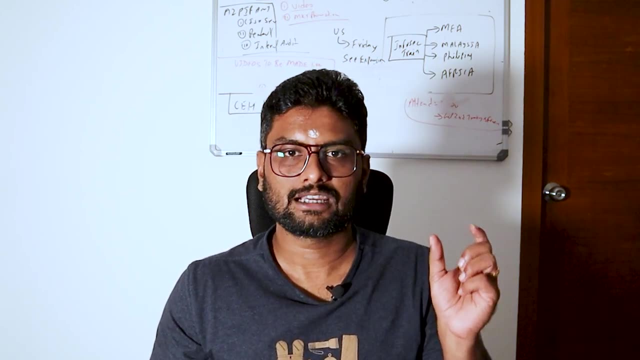 the organization in a negative manner. That is called as an incident. The every incident is an event, but not every event is an incident. Let me explain you. Let me understand the difference between the event and incident. I have a session. I have 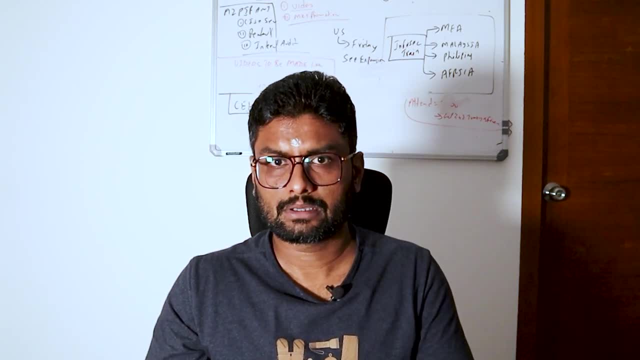 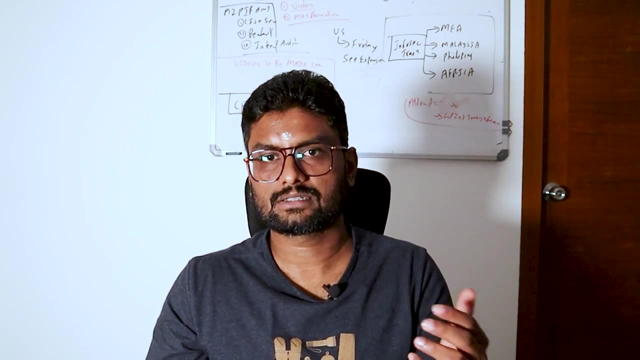 to start a session by 6.30 and I trigger an app and app open, initiate it at 6.30 and we start a session by 6.30, which is basically run as per the business objective. That is an event, But app doesn't trigger till 6.30, trigger by 6.40, I fail to continue it impact. 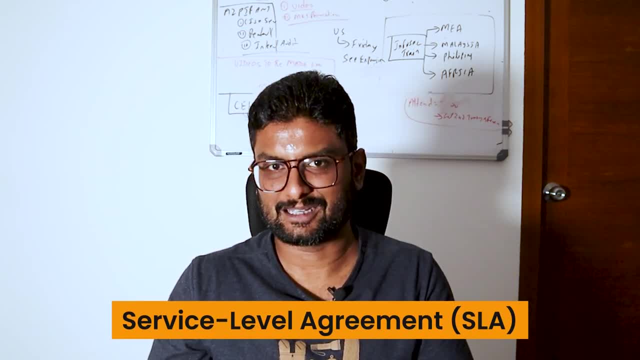 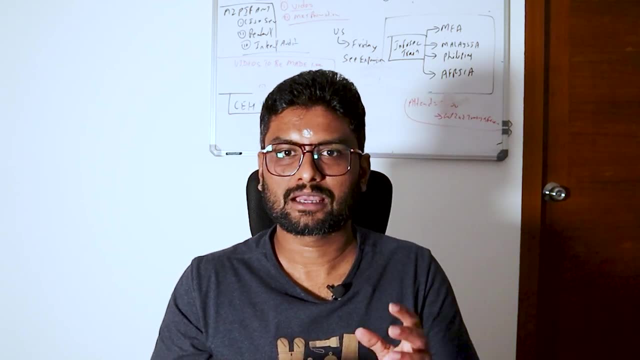 my CIA. Then it become an incident Because here we breach the SLA. That is the thin line difference: the event and incident You are attending. so your parents make you full makeup shake up, you make you ready to attend one marriage event. You're going with this impression: you're attending one marriage. 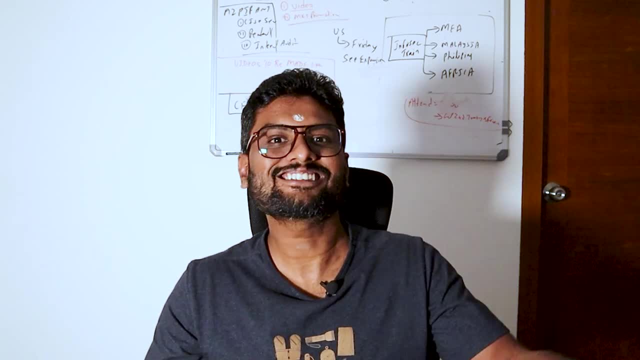 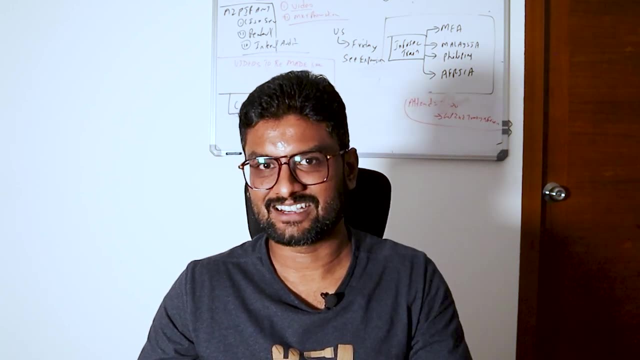 event and later on you got to know your marriage got fixed in that event. Then it has become an incident for you. Now you understand. So every incident is an event, but not every event is an incident. So let's start with the first part, which is basically called: 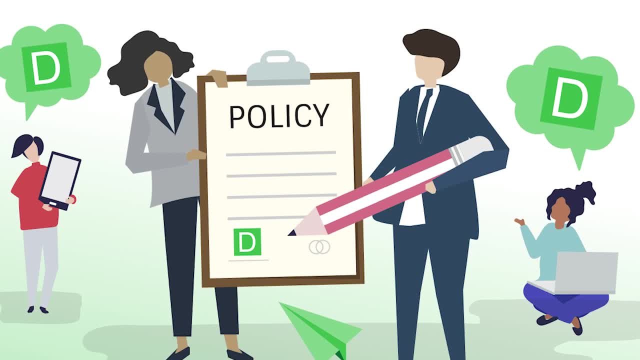 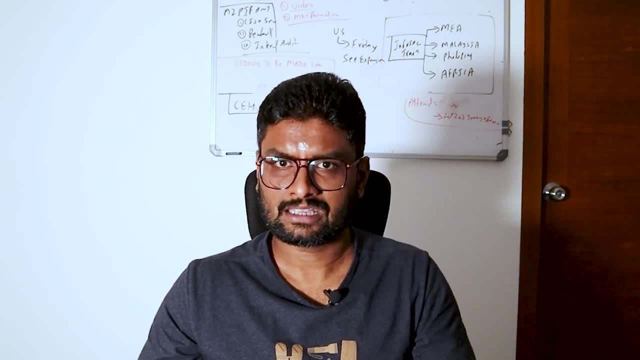 as a stage, Stage one, preparation In a stage one. the first step is called as a policy. Any kind of a system you are introducing in the organization, any kind of a system you are introducing in the organization. Okay, you need a policy for that. Okay, policy, basically, help me to. 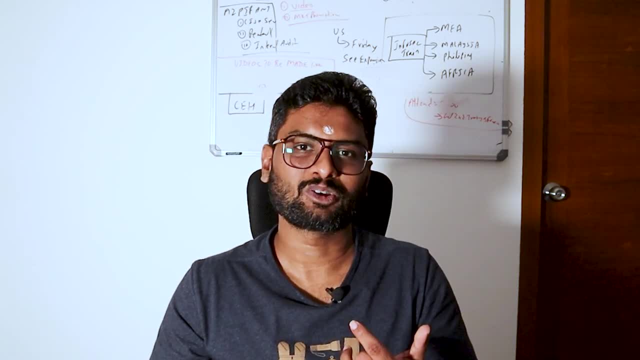 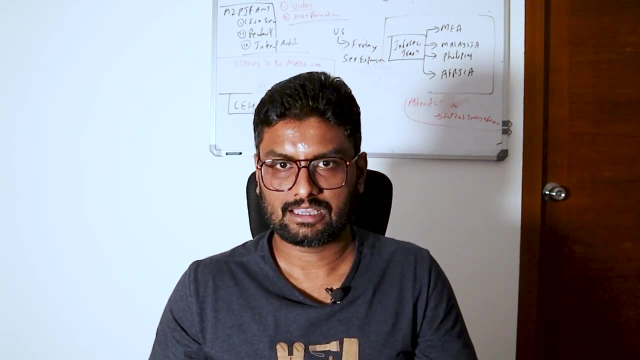 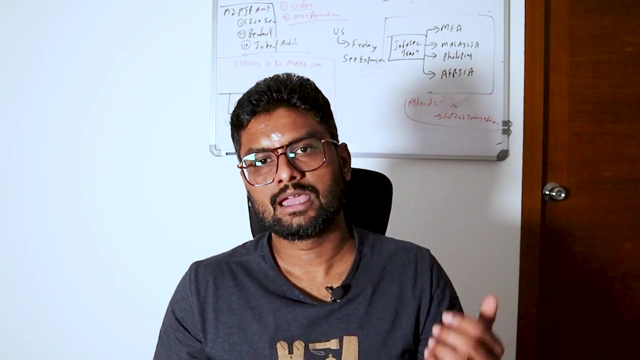 establish the governance Policy, talk about the scoping policy. basically talk about the structure policy, basically talk about the responsibility matrix policy, talk about the authority and all that. So it is created by the information security manager. It talks about why we need an incident management system in the organization And it is basically 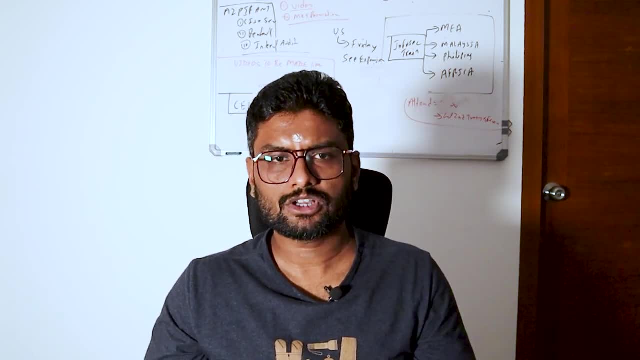 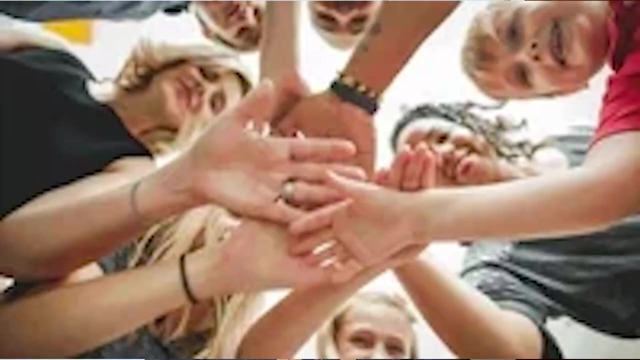 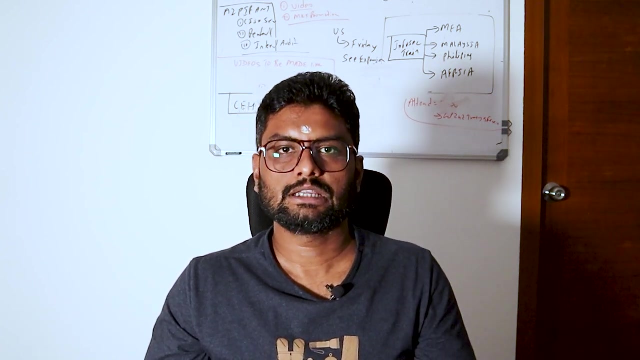 approved by the senior management. So once we have a policy in place, the second thing what we do is we create a team. we form the team which is called as a CSIRT team- centralized security incident response team. After having an incident response team, we'll basically. 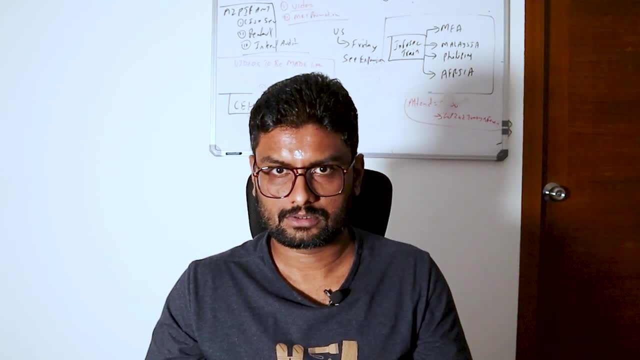 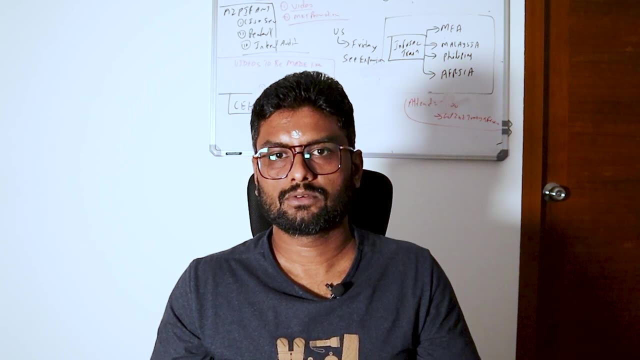 develop the plan, because it is very important to have a plan. It is very important to have a procedure in place. So, example, like I am the incident management lead and I am the one who created a plan, Now I am basically having an off In my absence if any incident happen according to the plan. 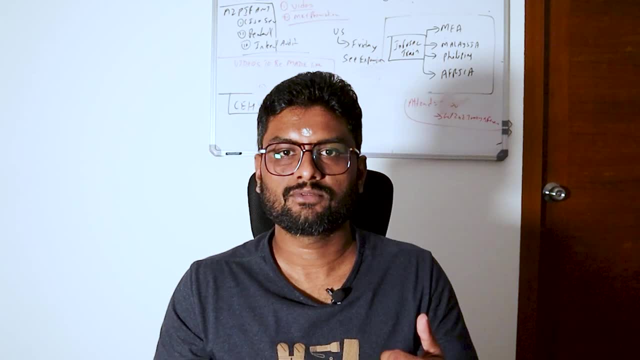 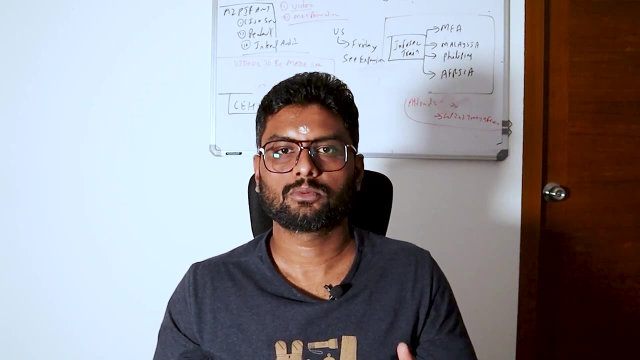 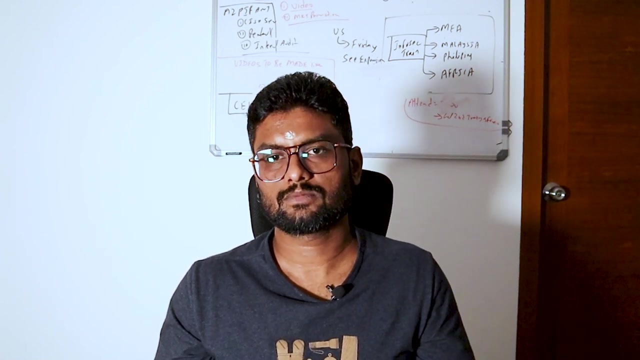 how to respond to the incident. it will be easy. That is why we need to have a good, detailed plan and their associate procedures. Once you have a plan, then you basically, based on that, you procure the tools, like we have a threat Intel, we have a SIM, we have IDS, we have antivirus, because these are the solutions. 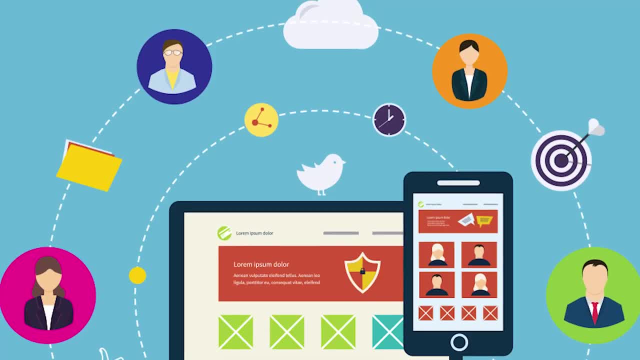 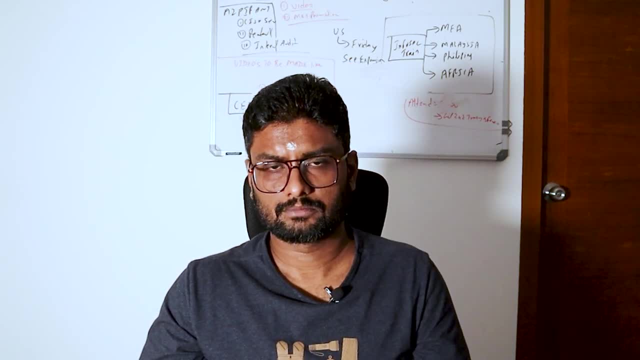 we have, which give the indication of an incident. Along with that, one more thing: what you need to consider is called as a train your employees by the security awareness trainings, because they are considered as a first layer of indication of incident and last layer of defense. 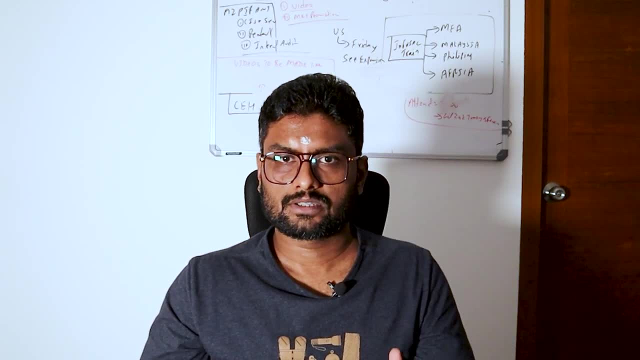 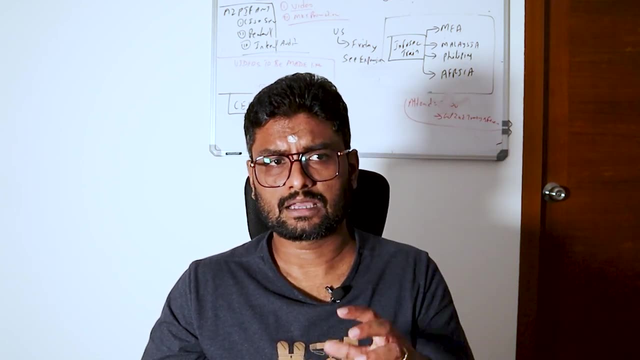 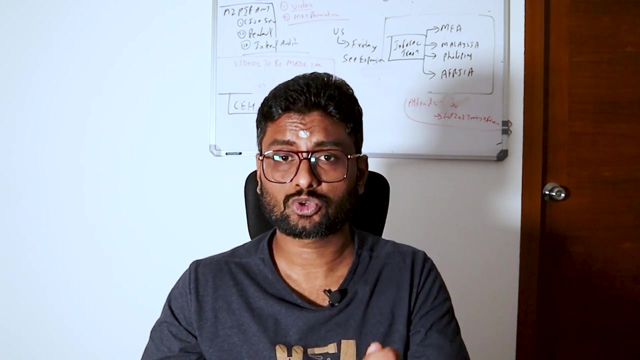 So we train them about what is security, why security is important, what is their responsibility toward the organization And how you measure the awareness training is like example: like before awareness training the people reported 70 incidents, but after awareness training they reported 150 incidents. that shows the good indicator of the security awareness. 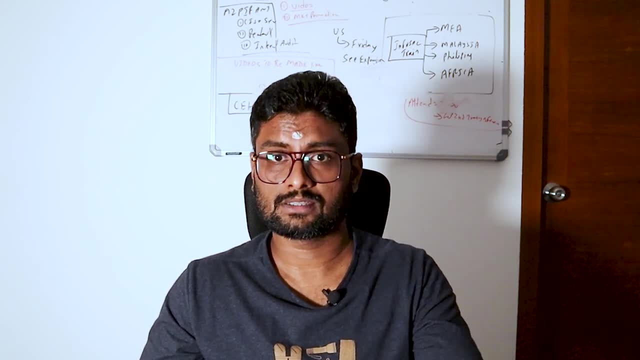 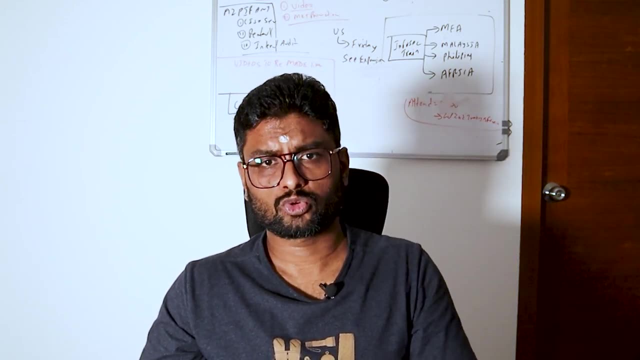 training, because now people are much aware about: okay, this is the incident, this is the symptom, this is the symptoms and all that. that is a different story. when they report an incident, It is not necessary, it's a true incident, but it is a good they have. 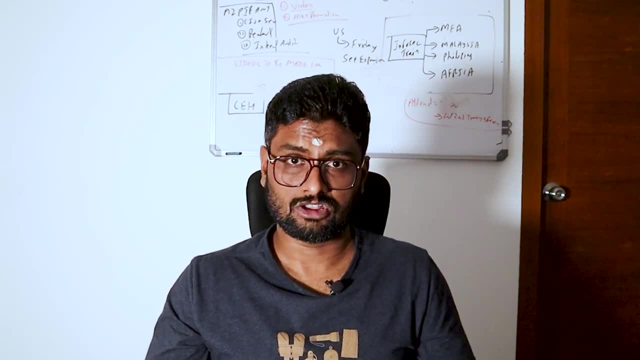 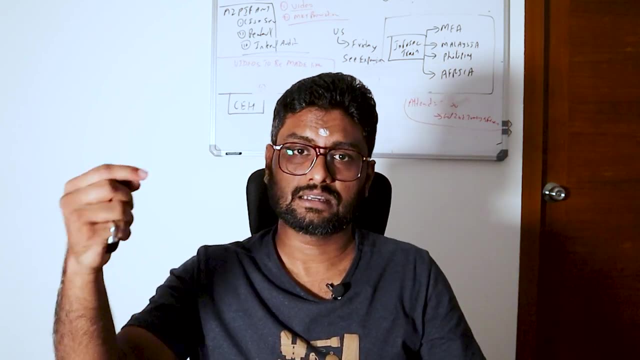 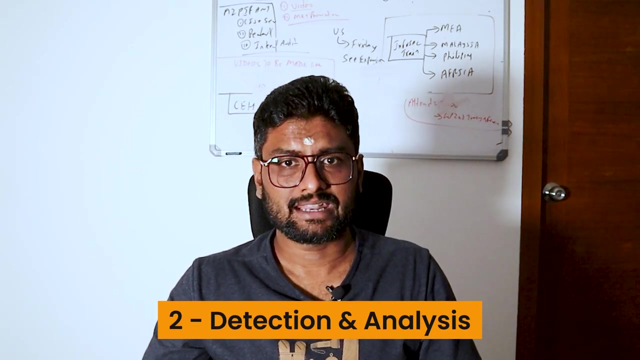 reported. So a good success factor of awareness training is increase in an incident report and decrease in a security violation. Okay, increase in an incident report and decrease in a security violation. So these things are what I have talked about in this video. I will cover the first two. 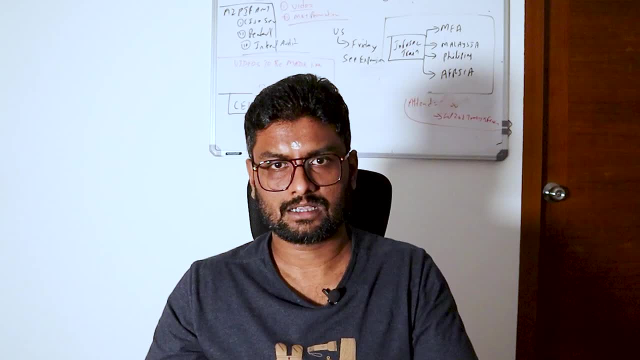 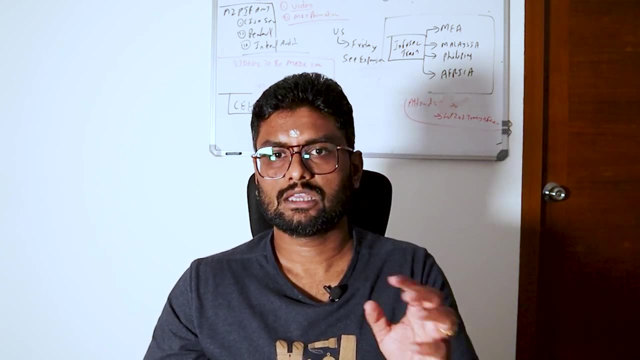 stages. first stage, which is what you need to know. The second stage, which is what I will do, is a very important small step in your life. And the second stage is called on the next stage. the first stage is called as detection. 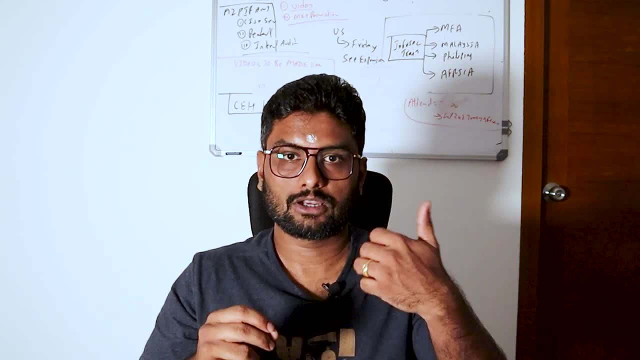 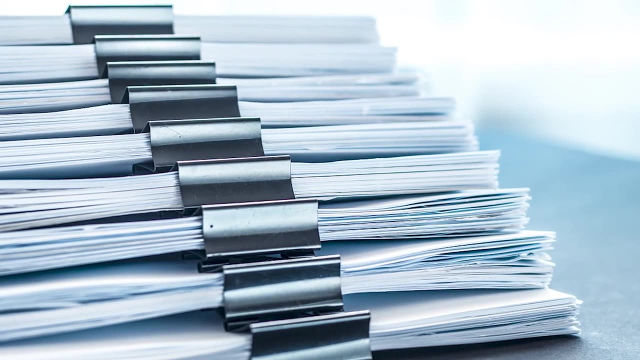 and analysis. So here one of the users has reported me a virus. There is a virus in my system, there was an attack, There was a breach in my system. So here he reported me. as I said, it is not necessary. Whatever he reports, it is true. 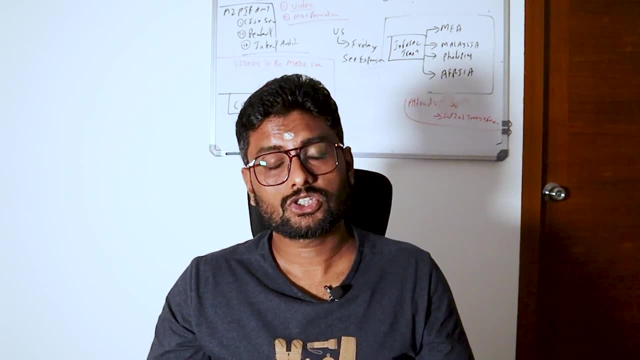 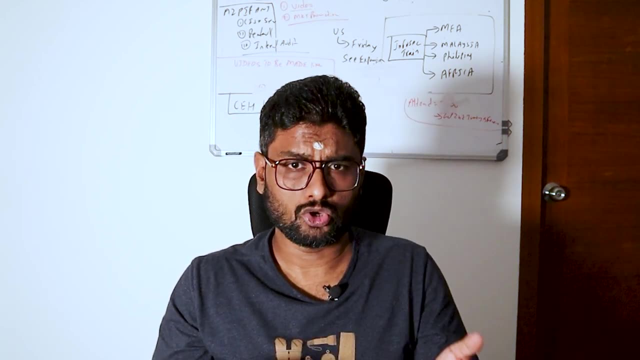 process because it has helped me to build the governance. so once you have a documentation, you will prioritize the incident. because you receive multiple ticket. it is not possible for you, as a human being, to report all the incident and manage all the incident, respond to all the incidents. 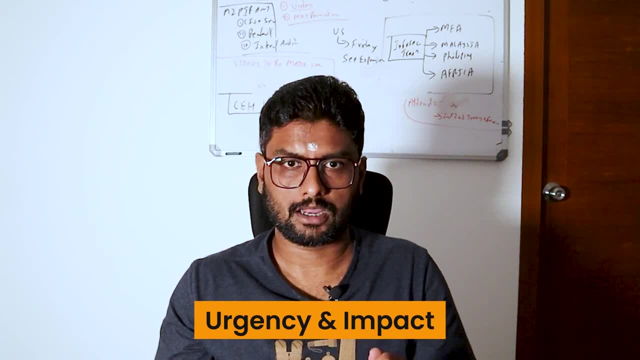 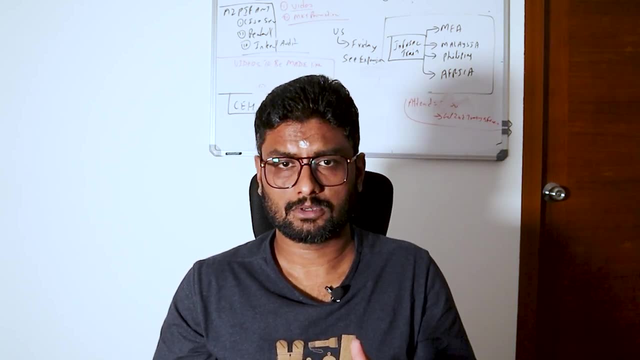 so you will do the one factor here, which is called as the urgency and impact same. like during a covid time when we have a mass patients in the hospital, it is difficult for the doctor to handle each and every patient on an individual level. so what they did, they did the urgency impact analysis. 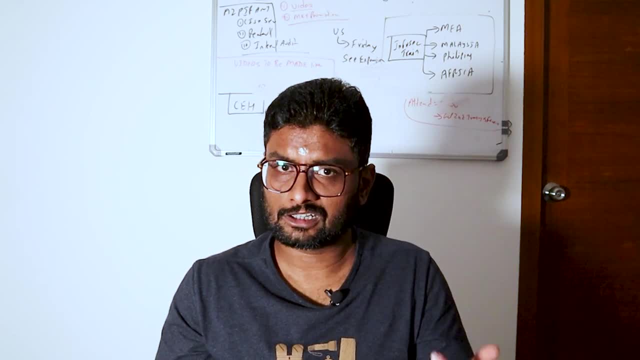 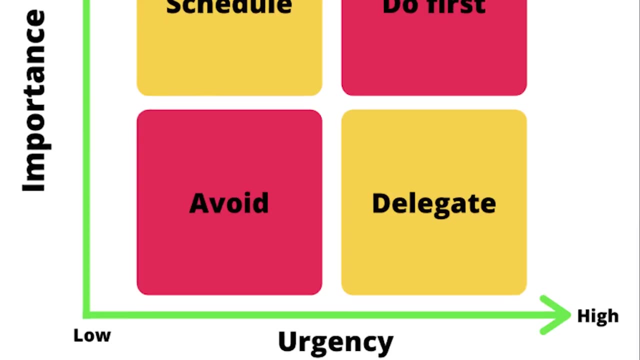 and identify which patient is critical and according to that, they have treat the patient. same thing happened here also, we have a multiple tickets. it is very difficult for us to manage the ticket. so what we did is we prioritize and we check the urgency impact, like which is which? 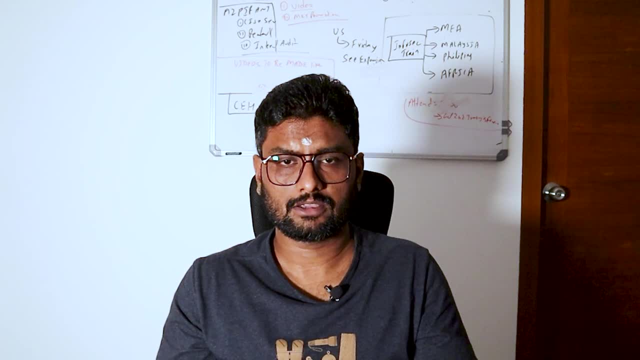 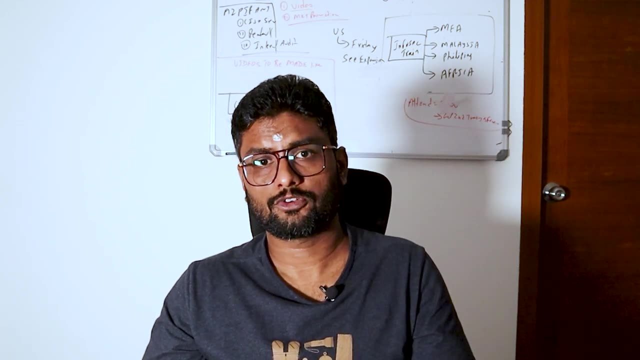 incident is basically urgent, which required urgent treatment. if i don't treat them, what is the impact? so that is how we basically did the impact: privatization- and according to that, we have notified the respective owners. now, example like this is a security breach and as for the regulatory, 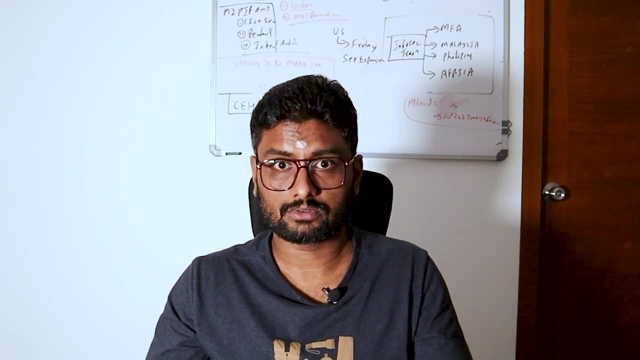 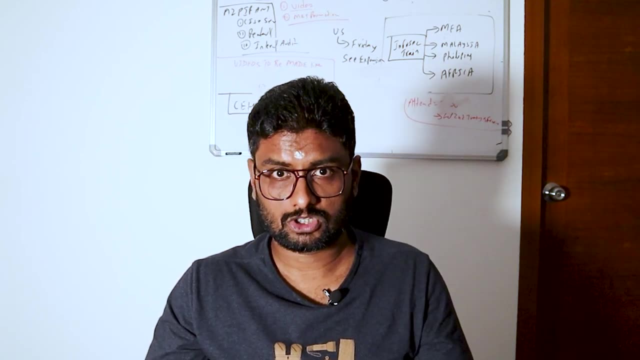 requirement. we need to report the breach to the government in 72 hours. like in gdpr, we have a reporting breach is 72 hours. in india we have a six hour, so we have to report this breach according to this timeline. so this activity is part of a detection and analysis. now next, 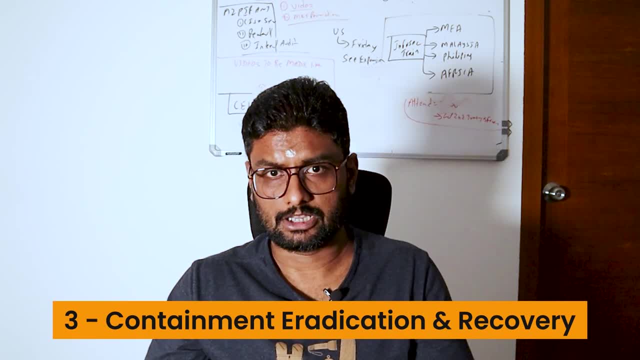 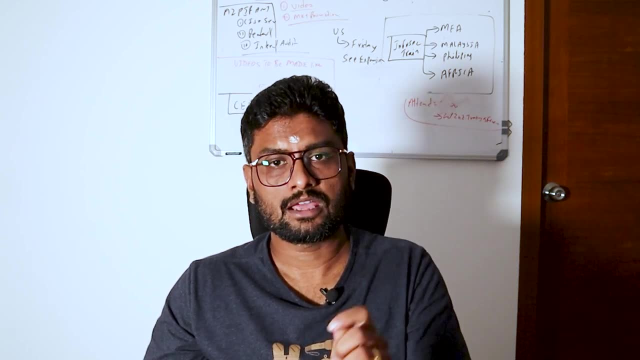 is called as a containment, the stage three, which is called as a containment, eradication and recovery. containment is all about limiting the impact. eradication is all about removing the impact of the impact. eradication is all about removing the impact. eradication is all about removing a threat from a system, and recovery is restore the system back to the production. so when we're 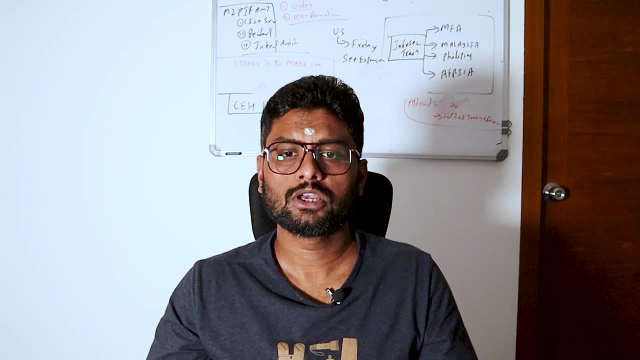 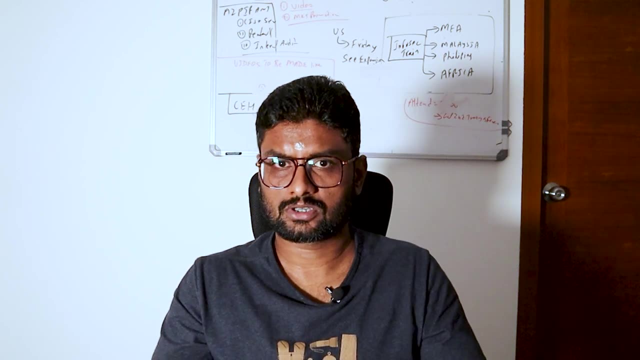 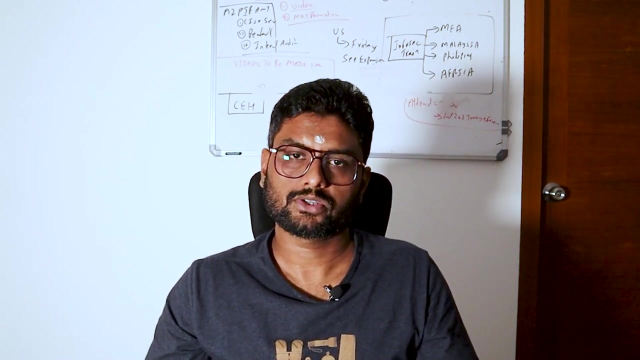 talking about containment, eradication, recovery. the first part we are doing is we are reporting. detailed reporting we are doing. we're preparing a continuing strategy how to contain the virus. example: system was infected with the virus. we know that. we confirm that. isolate a system from the network: that is my first priority. isolate a system from the network: that is my first priority. 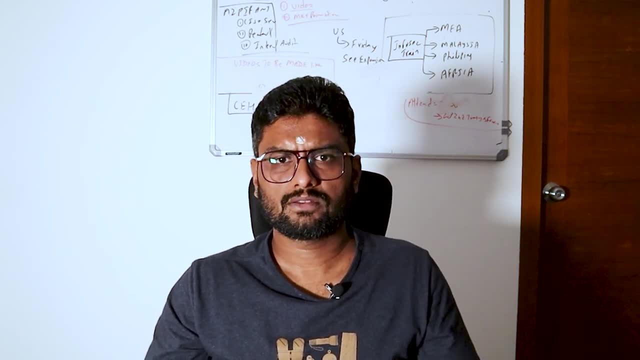 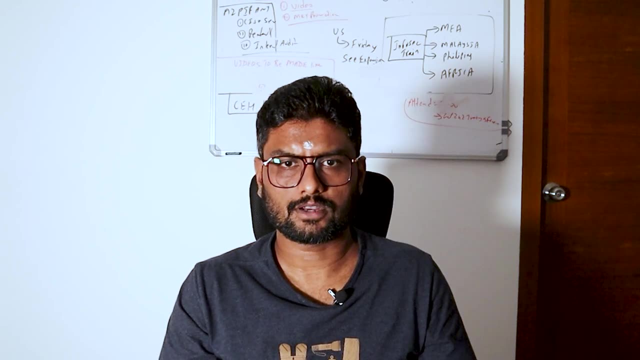 that is the first thing we do in a part of a containment seem like. you know, when we have found some covet symptoms and all that, we isolate the person immediately from the family. right, the same thing happened here. so system was infected with the virus. the system is hacked, batteries isolate. 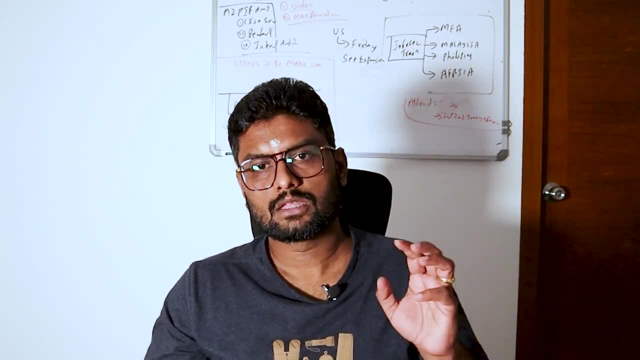 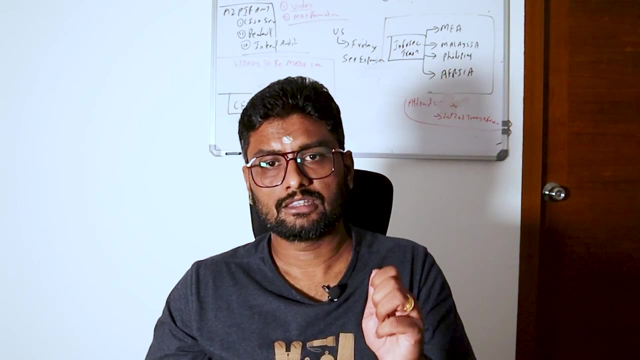 a system from the network. that is a temporary best solution. then we try to remove all the threat from a system, like if the system was infected with the virus: remove the virus from the system. okay, then we did do the detailed reporting and notify my senior manager or manager, because sometime what? 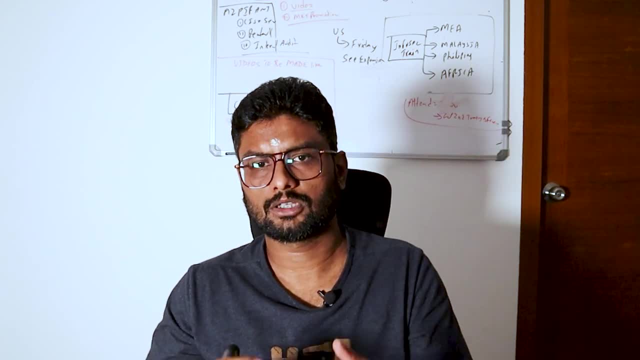 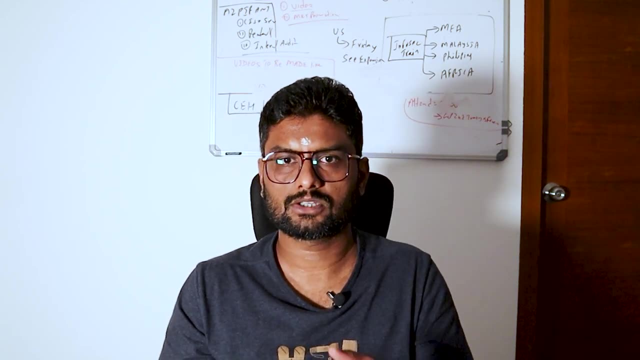 happened. restoring a system, removing something, installing something required a lot of cost. if you required the budgetary approval, you will notify and because sometime what happened when you isolate it impact the availability. so we need to see the business impact analysis. so we'll review the bia to. 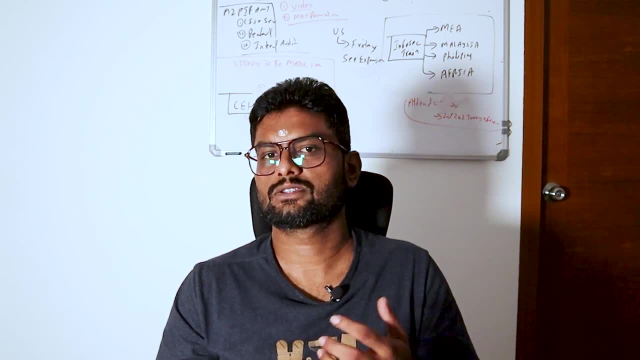 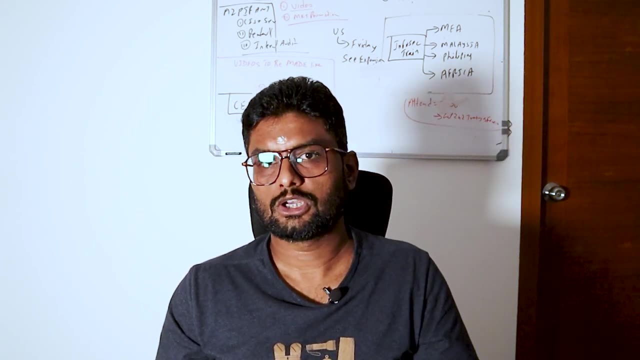 understand which business is critical: is the process which is running on this it is critical or not, and according to that we perform the recovery where i restore the system back to the production. here, one thing we need to notice is when we're restoring a system back to the 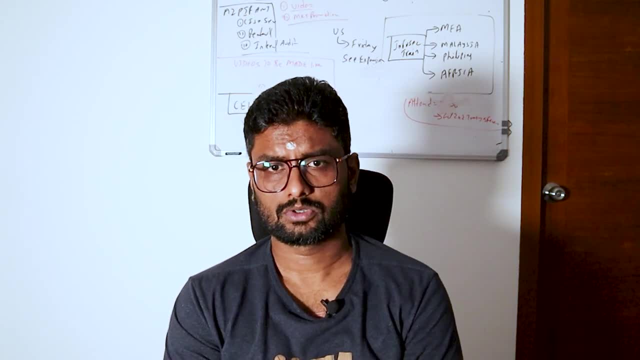 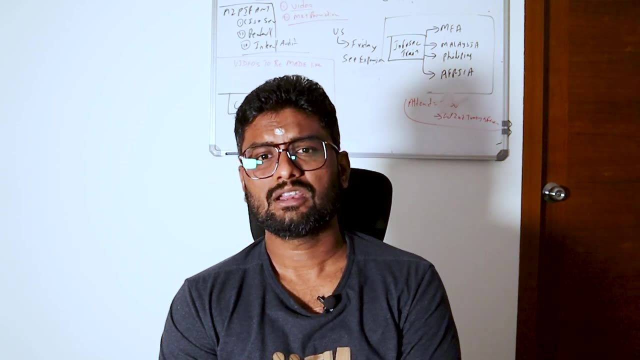 production, we have to restore within a defined mtd, rt and rpo. and as for the sla, so now i'm assuming the system was a restore as per the bia, there is no breach of sla. now let me learn how this happen. what is the reason of this is?